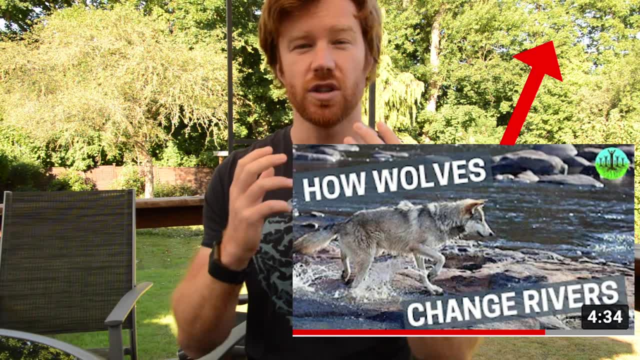 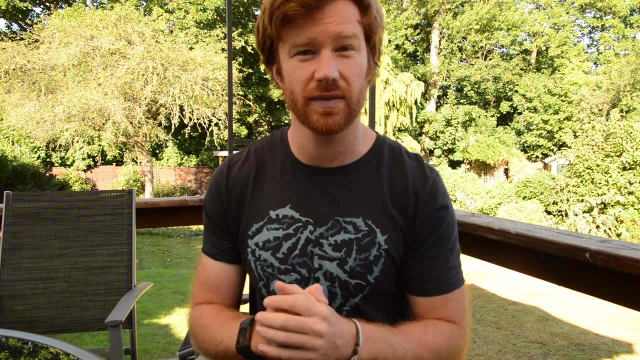 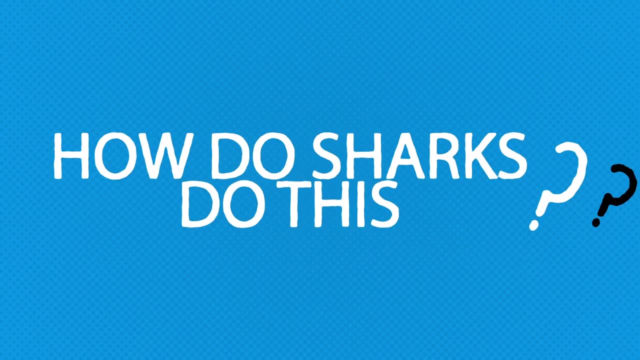 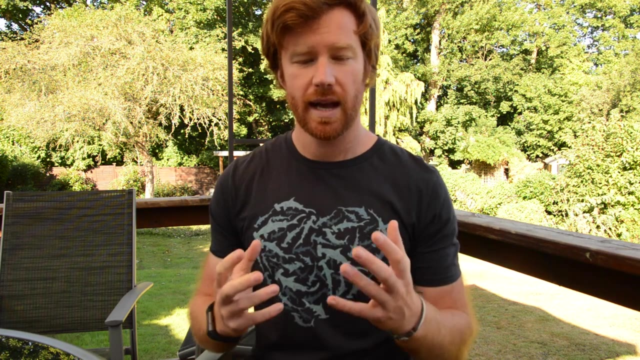 go watch wolf change rivers before continuing this video so you can get a really good visual representation of how keystone species can impact the whole environment, from the smallest of animals up to the biggest of trees and the whole ecosystem, and how it works. So how does this work for sharks? How are sharks keystone species? Well, as I mentioned, 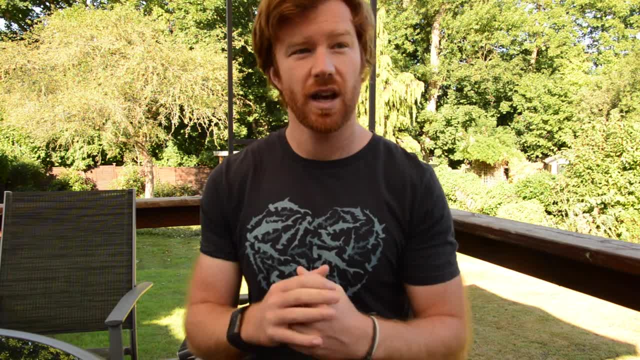 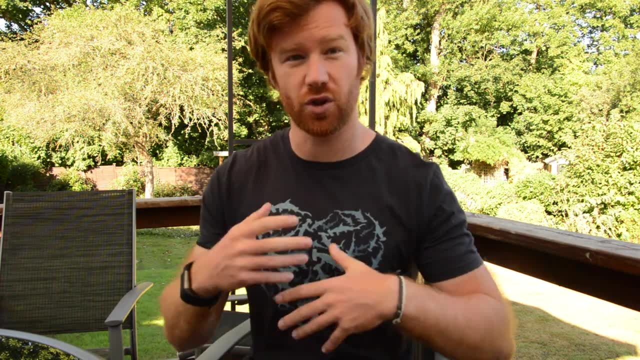 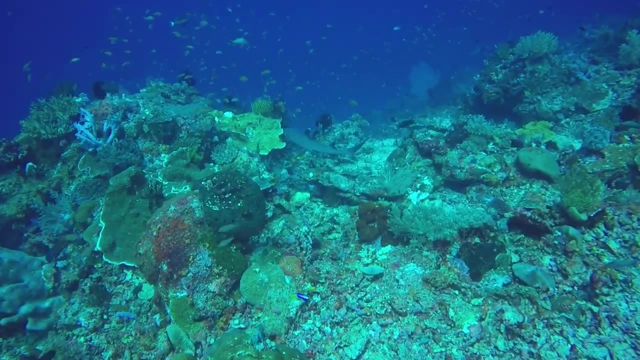 sharks are apex predators and therefore they hunt a number of different fish and other animal species in the ocean. Now, by hunting all these different species and constantly putting some predatory pressure on these different species, they stop any one species overpopulating, So they don't allow any one species just to grow out of control and therefore 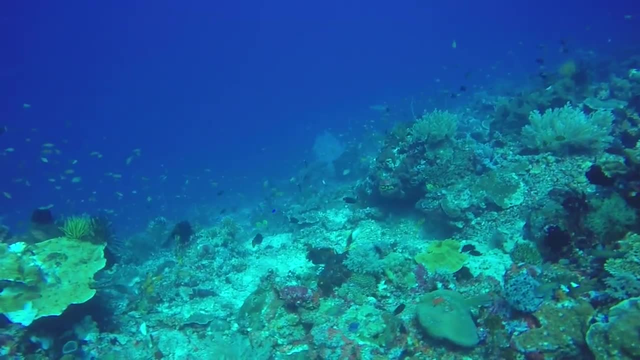 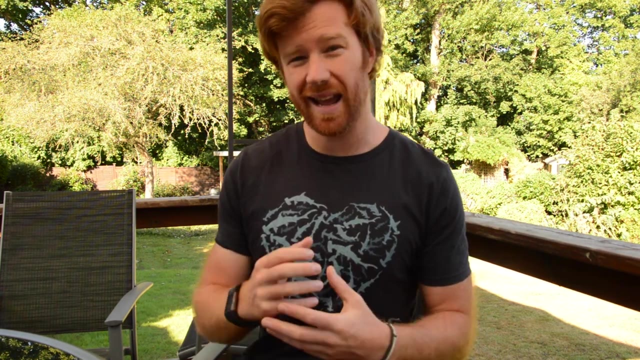 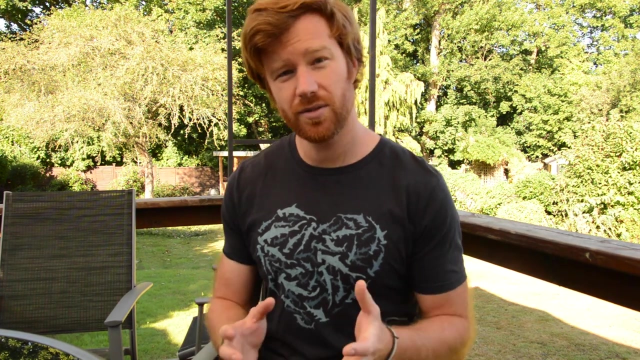 take over a whole ecosystem, like we saw the deer had done in Yellowstone National Park. They also maintain the health of the ecosystem by hunting the dying and the ill fish, and this actually stops the spread of disease reaching through a whole population. So how does this affect us? You know a lot of people might say that the health of the oceans 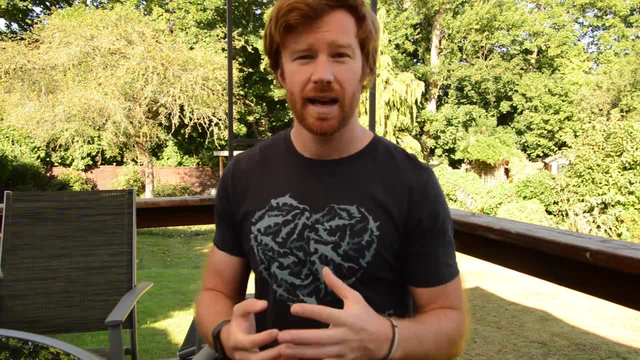 doesn't really affect us on land. we don't live in the oceans. however, healthy oceans provide up to 85 percent of the oxygen that we consume. So how does this affect us? Well, as I mentioned earlier, sharks are apex predators and therefore they hunt a number of different species in the ocean. 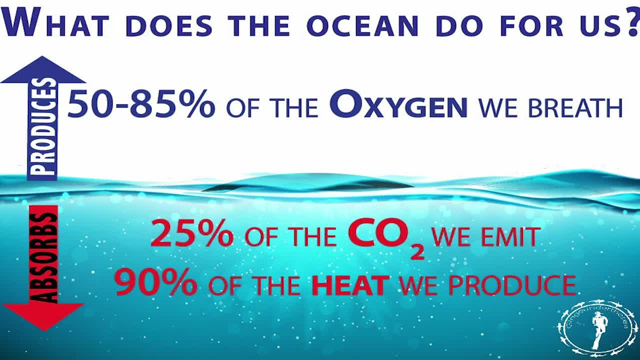 So this means that every other breath that you take actually comes from the ocean, So we must have a healthy ocean ecosystem in order to have the oxygen that we need to breathe. The oceans also store 25 percent of the carbon dioxide that we produce through carbon emissions. 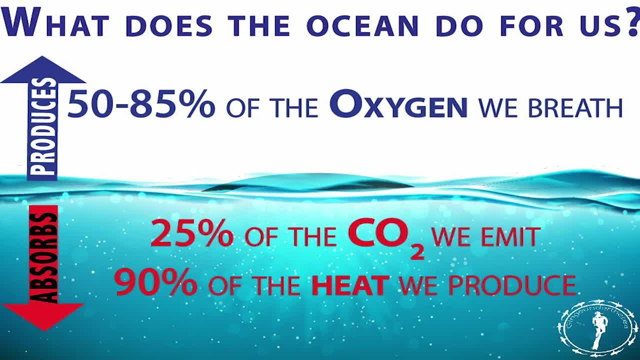 which is a massive amount, and also they absorb 90 percent of the heat that we produce through carbon emissions as well. So basically, without healthy ocean ecosystems, sharks are apex predators- We would be living on a very hot, very oxygen, poor planet that just would not be suitable for human. 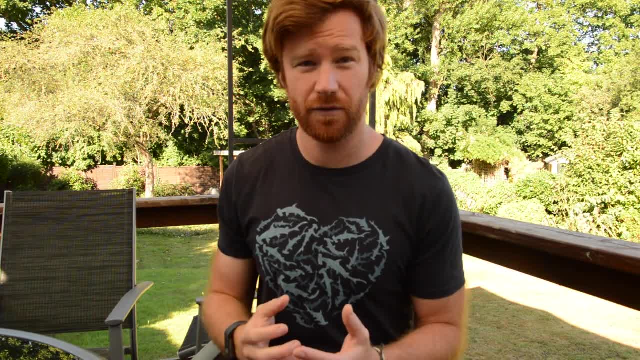 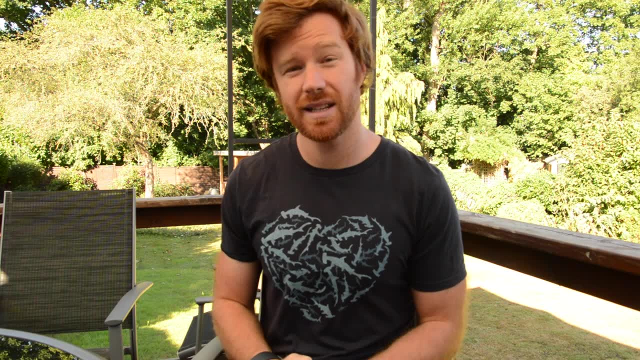 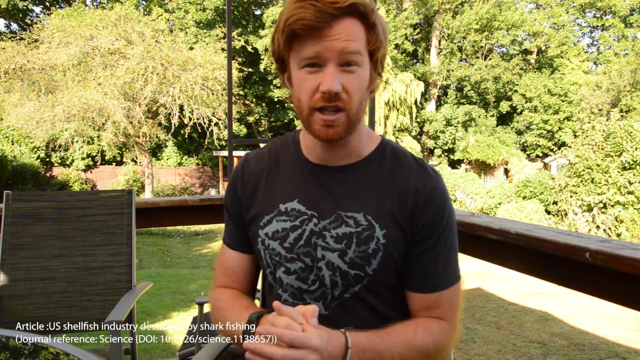 life, And if we want to look at a more direct effect of sharks on the ecosystem that will affect us, we just need to look at a study that was published in 2007 looking at the impact of the decline of large print sharks on the shellfish industry on the east coast of the USA. Now, 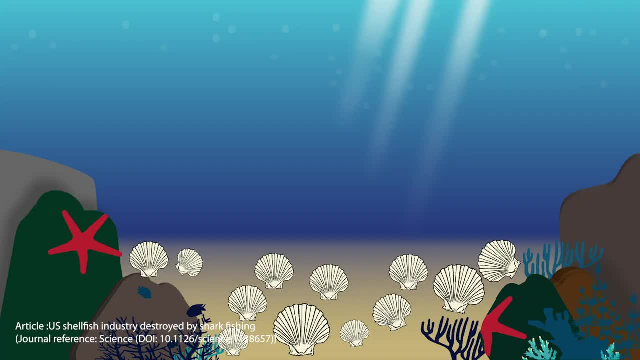 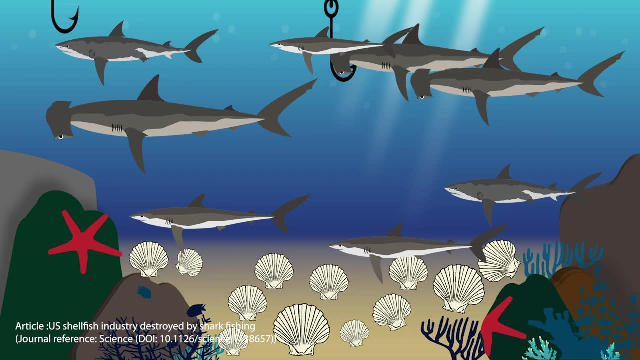 this study found that there was up to a 99 percent decrease in just 35 years of many of the large predatory shark species, such as dusky, smooth, hammerhead, bull sharks, scalloped hammerhead- these very large predatory species. they were declined by 99 percent in some areas And with this decline, the prey species of the 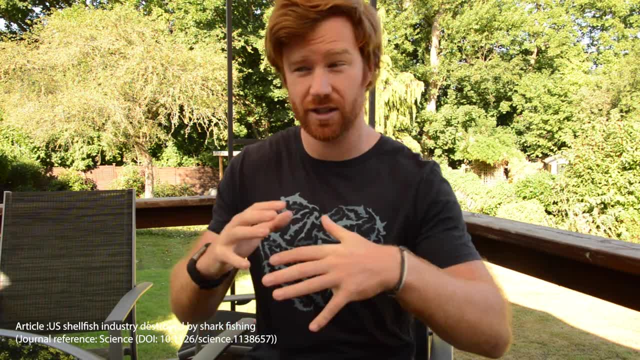 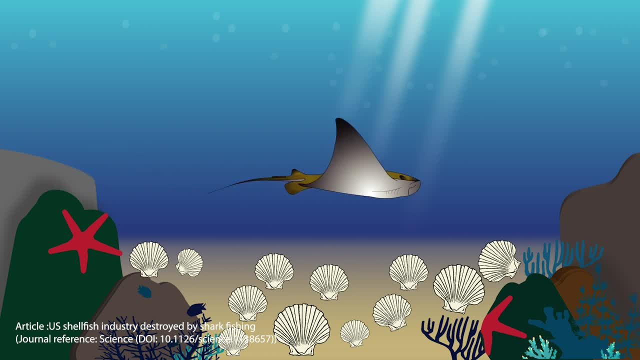 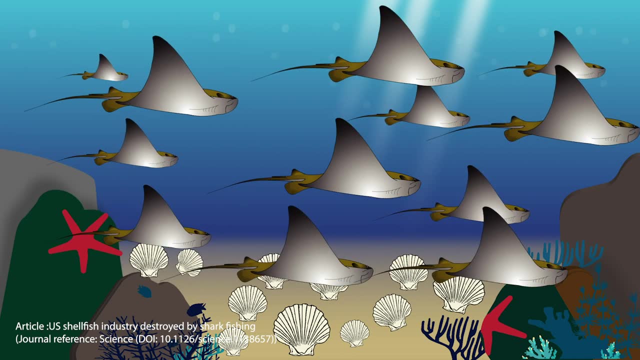 sharks obviously could rise unchecked and just grow out of control, and one of the species that benefited most was the cow nose ray. And so, again, this study predicts that the cow nose ray increased in population by tenfold in this 35 years, which is extremely fast for a species that has so low productivity And with this huge 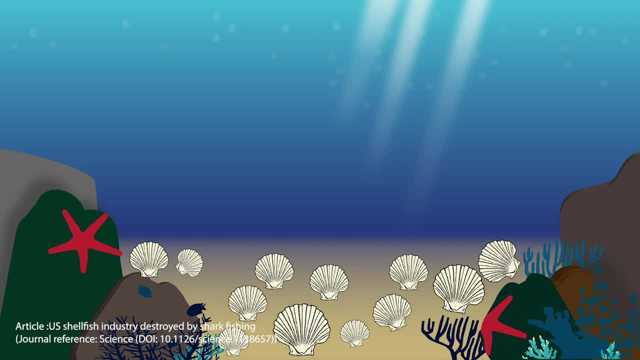 increase in biomass of cow nose rays. their prey source, which was the bivalves and the scallops, actually were completely eradicated in that area due to the over foraging of the cow nose rays, and this impact was emphasised as as soon as you move out of the range of these cow nose rays. 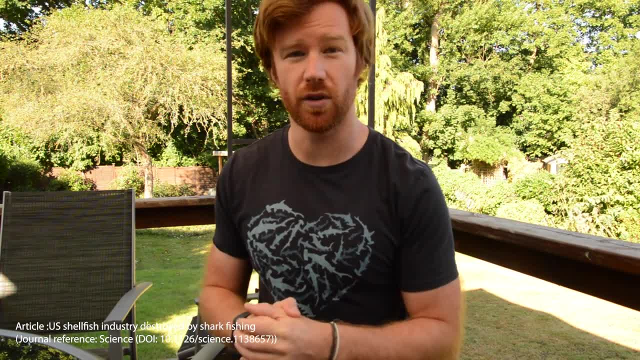 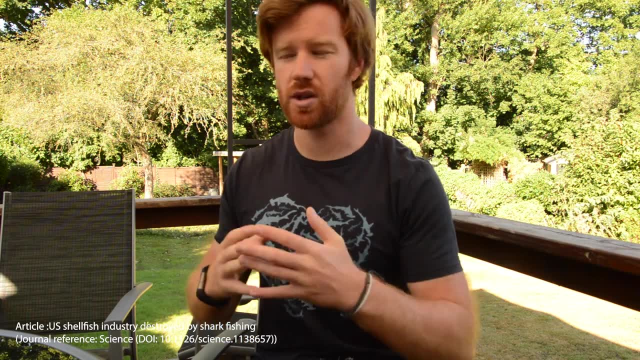 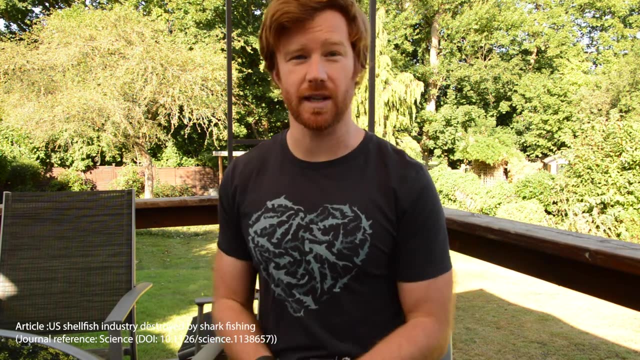 the shellfish industry was doing fine and actually numbers of mollusks were increasing. But as soon as you go within that range of the cow nose rays, the shellfish industry was just collapsing because there was just no shellfish left, as these cow nose rays were just over predating and removing all of the mollusks. So we can see how. 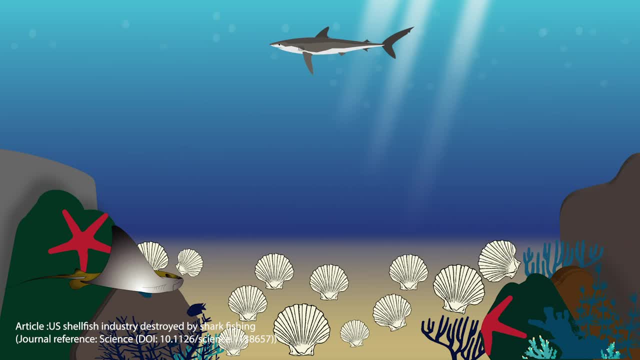 without predatory species, that in fact, there was a decrease in the number of mollusks that the shellfish industry was able to get rid of. In fact, there is a chain reaction that means that actually our own industries can be impacted by it, And so this brings us on to the economic impact of sharks. So 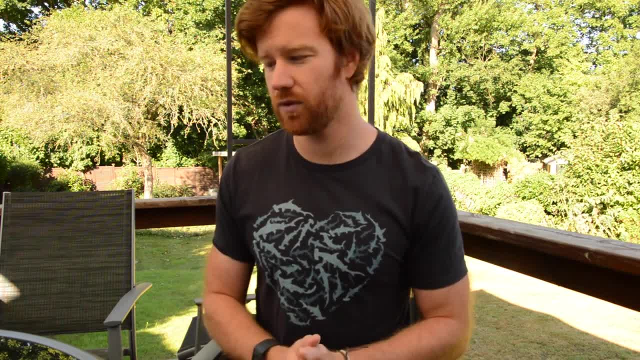 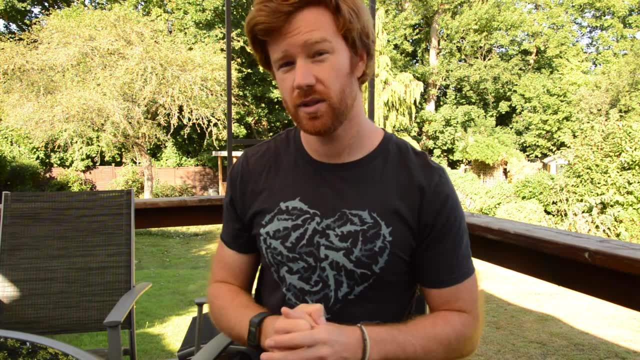 not only do sharks help keep our fisheries healthy, as we've just shown in the study before, but also they directly bring money in through shark tourism. As an example, Bahamas is reported to have brought in over a hundred million dollars each year through the shark tourism industry alone.